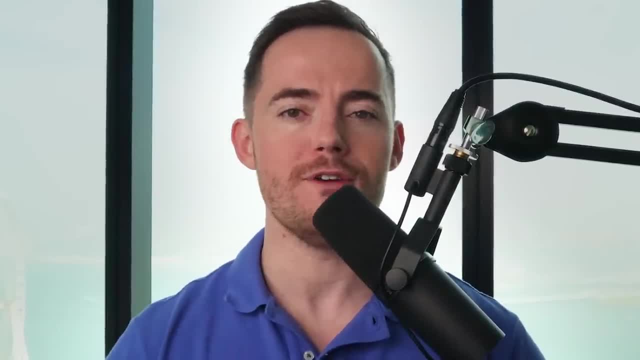 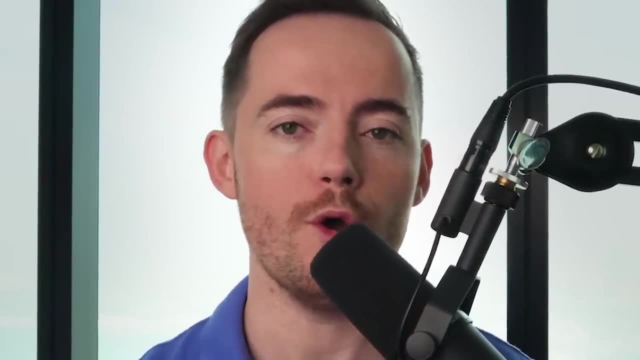 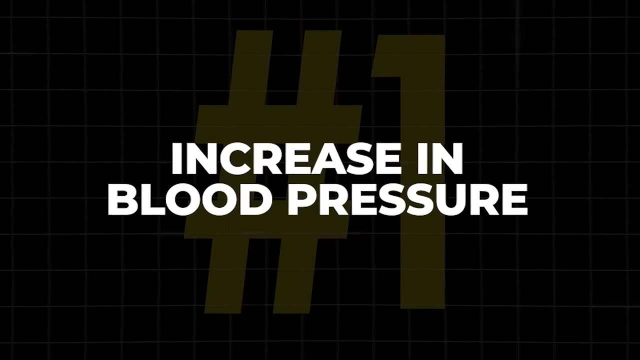 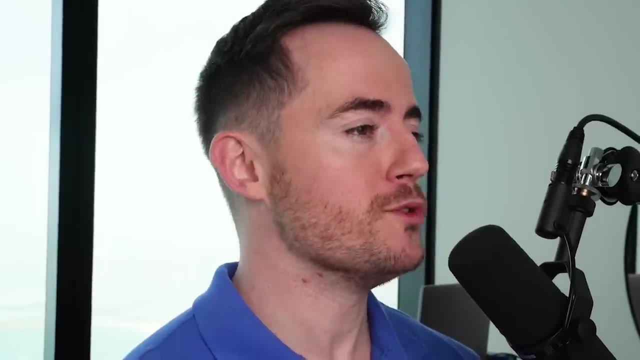 my breakthrough method or without AA willpower, rehabs or medication. I've taught this to people from NASA, PayPal, Forbes and Google. So the first sign is an increase in blood pressure. You'll often hear blood pressure called the silent killer, And for good reason. It often has no visible symptoms And the only 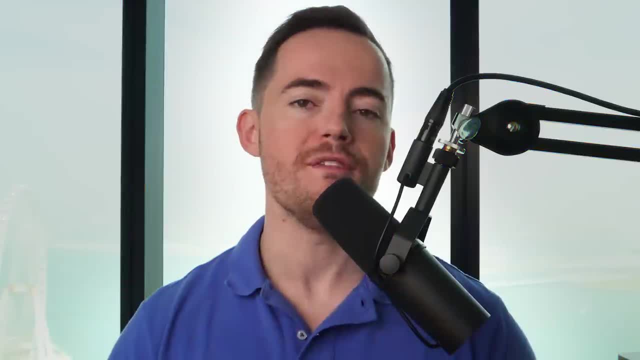 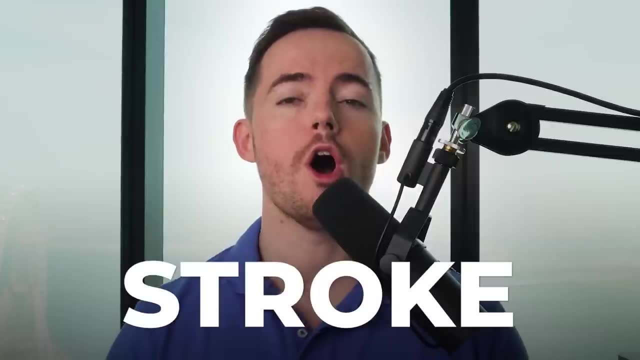 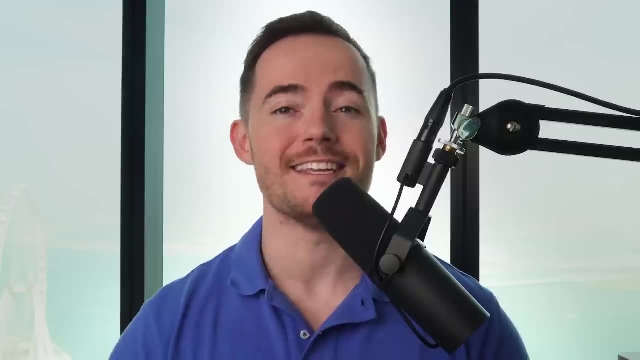 way to find out is to actually measure your blood pressure. But don't be fooled by this. High blood pressure dramatically increases the risk of death from other conditions, notably stroke, heart disease and heart failure. The CDC estimates that over 350,000 Americans die each year as a direct result of high blood pressure. If you want to live longer and healthier, one of the best tried and tested ways is to keep your blood pressure low. Unfortunately, elevated blood pressure is one of the first health effects of regular drinking. Compared to non-drinkers, women who drink double their risk of hypertension. 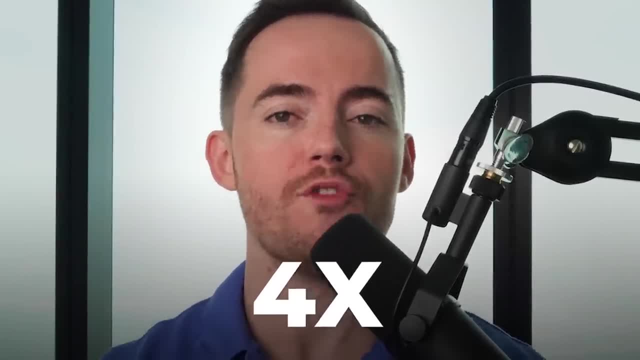 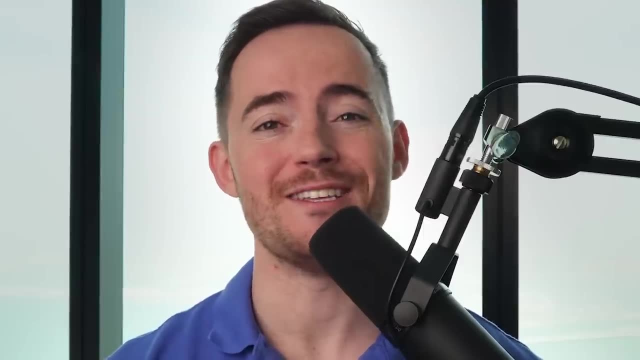 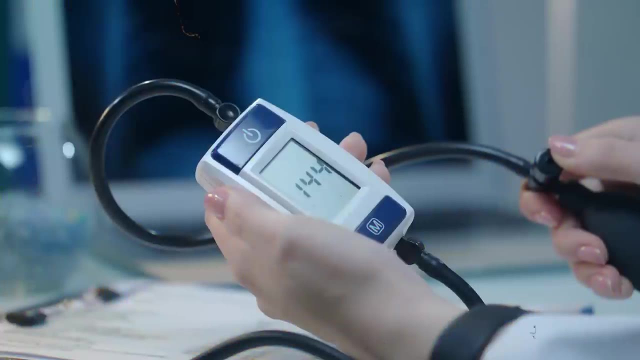 And male drinkers raise their risk by a whopping four times. Scientists call this condition alcohol-induced diabetes. It's one of the first and most certain signs that you have started to drink yourself to death. The good news is well, there's actually two pieces of good news. Firstly, checking your 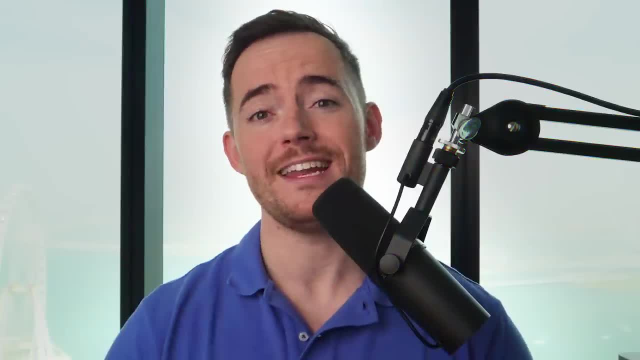 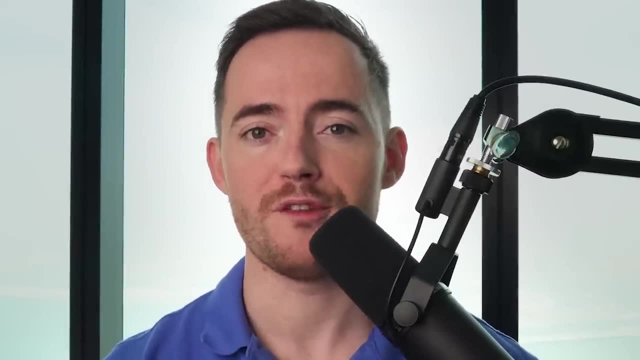 blood pressure is the easiest thing in the world, So if you're in any doubt, get it checked today. Secondly, there is a very effective way to reverse alcohol-induced hypertension. Are you ready for it? It's to stop drinking. The second sign is in weight gain, So it's related to blood pressure. 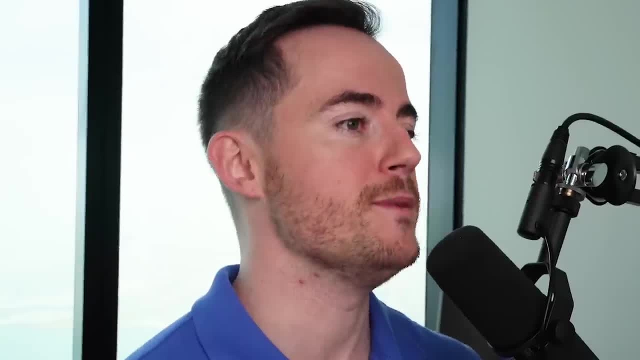 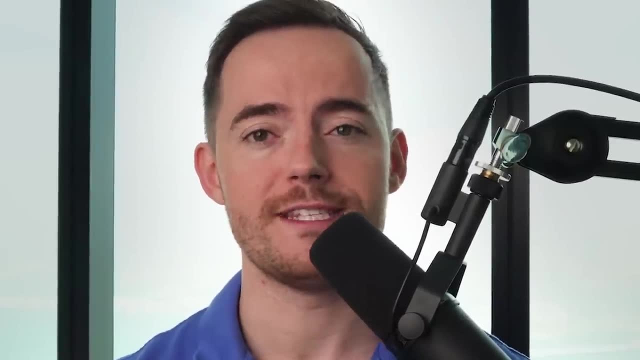 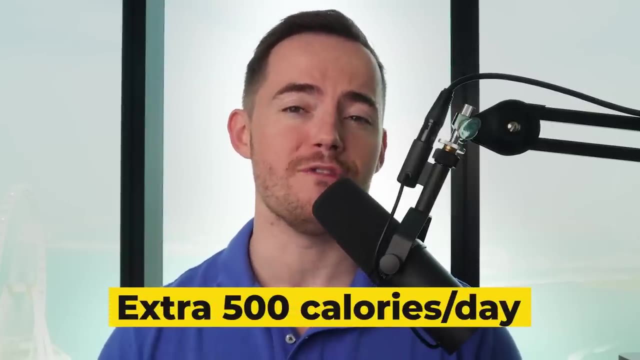 but alcohol is. nutritionally it's the ultimate junk food. Actually calling it a junk food is generous. It's really a mild poison, but still it's loaded with calories, typically between one and 200 calories per drink. If you only have two or three drinks a day, you could be looking at as much as an extra 500 calories. 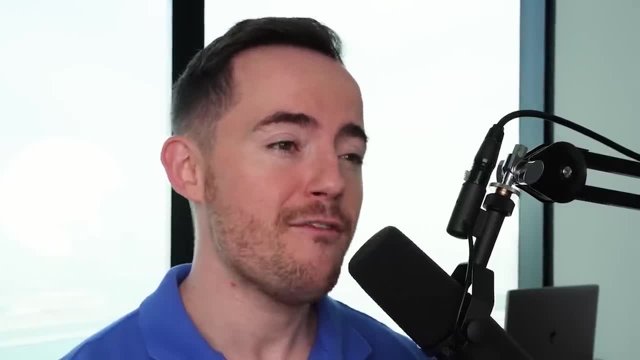 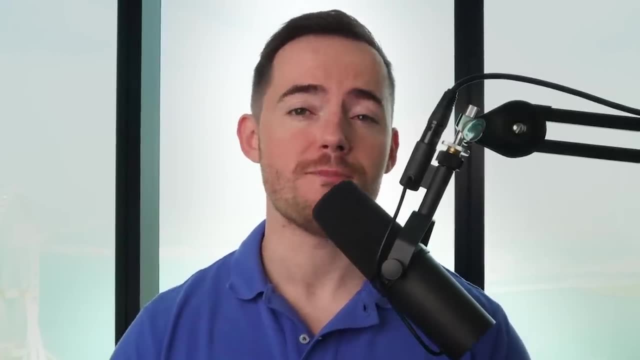 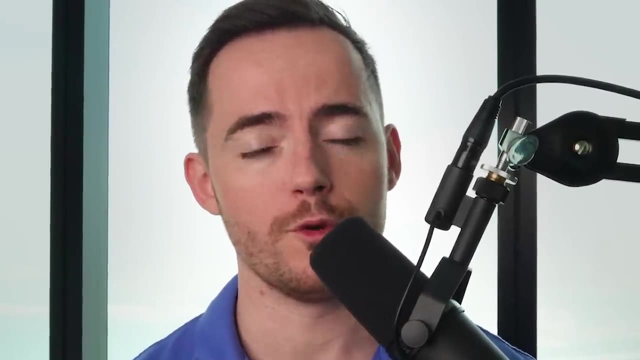 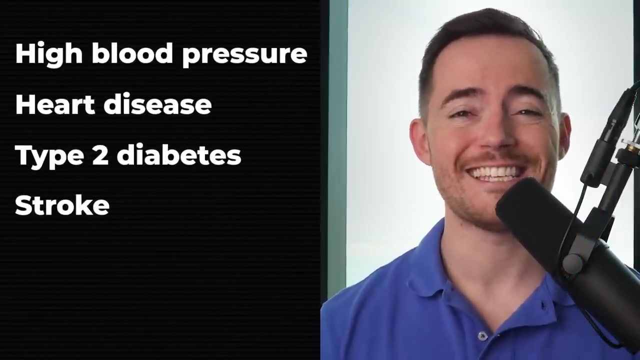 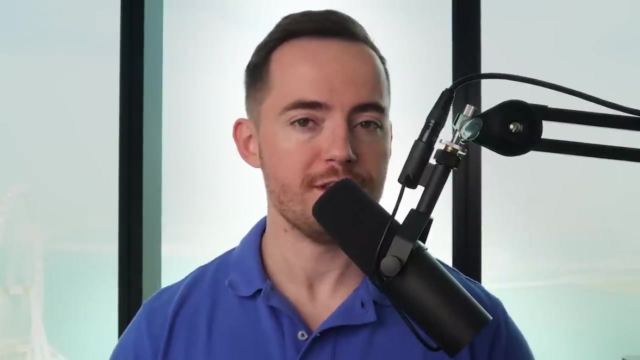 And even though alcoholic drinks are packed with calories, the ethanol will actually boost your appetite for even more food. Scientists aren't sure exactly why it does this, but they suspect it affects our hormones that regulate our hunger. The third sign is in memory loss. Alcohol affects cognitive functioning in all sorts of ways In advanced stages it can actually lead to full blown dementia- so-called alcohol related dementia- But this is late stage alcoholism. One of the first and most conspicuous effects of alcohol is the signs of memory loss. Health and memory loss can cause a lot of trouble. 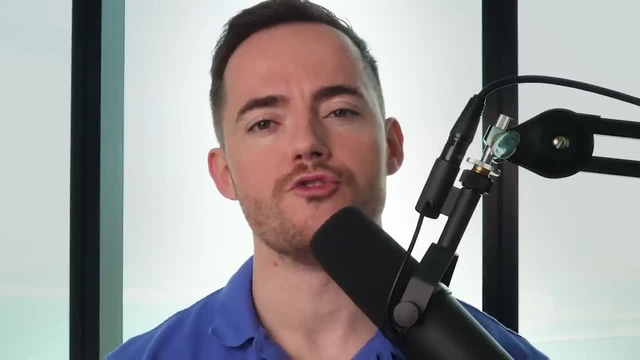 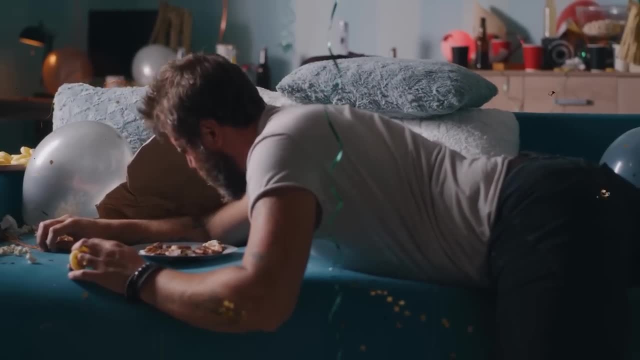 is on memory. Memory blackouts are one of the hallmarks of binge drinking. These are periods in time when you are heavily intoxicated and remember nothing. Other times the blackout is incomplete and you can recall fragments of what happened here and there. What's scary is that the 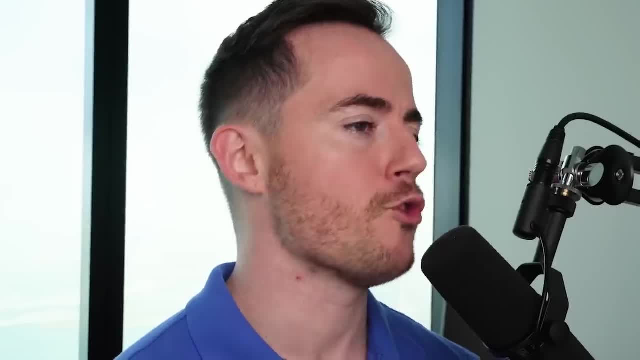 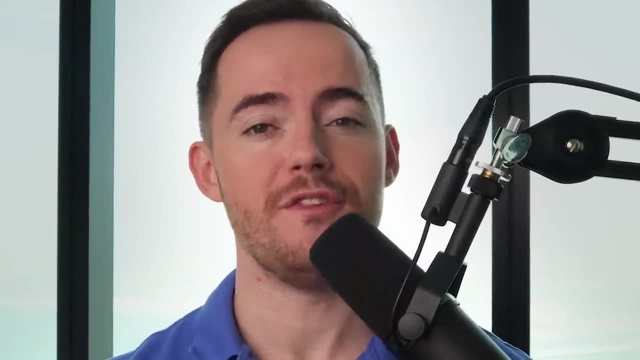 blackout isn't related to periods when you were passed out. Quite the contrary, you were wide awake and interacting with people around you, But you were drinking so heavily that the alcohol interfered with your mind's ability to form and maintain memories of that time period. These 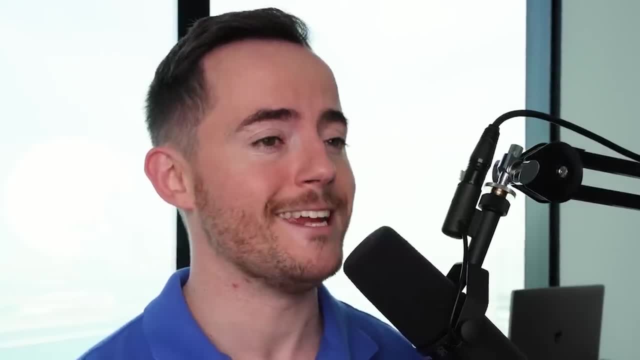 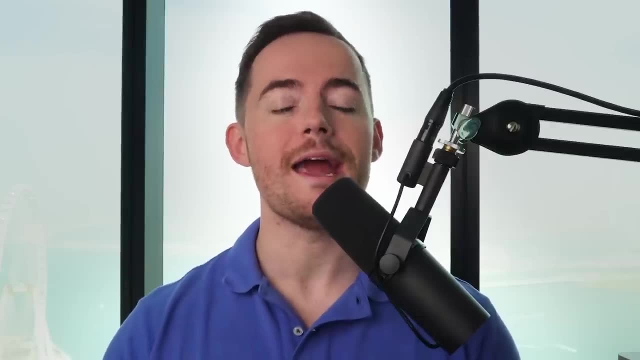 blackouts are a very conspicuous in-your-face sign that your drinking is getting out of hand. But what is happening at the same time is that alcohol is slowly but steadily eroding a wide range of cognitive functions. These include attention, decision-making, motor speed. 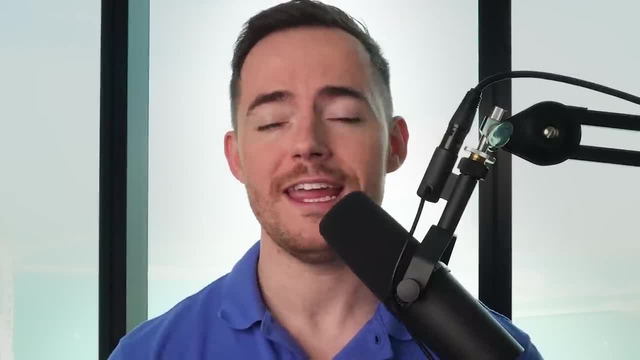 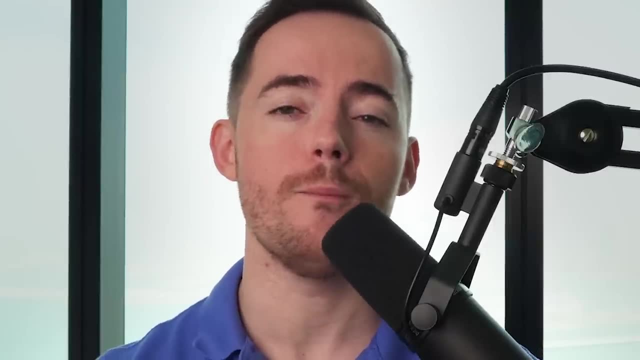 emotional processing, as well as more or less all aspects of memory, including working memory In late-stage alcoholism. it is hard to find a single cognitive dimension that can be used to determine whether or not you are drinking. The fourth sign is a change in appearance in your face. It's another big red flag. 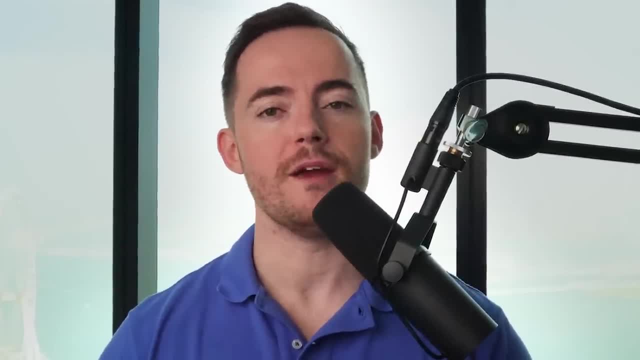 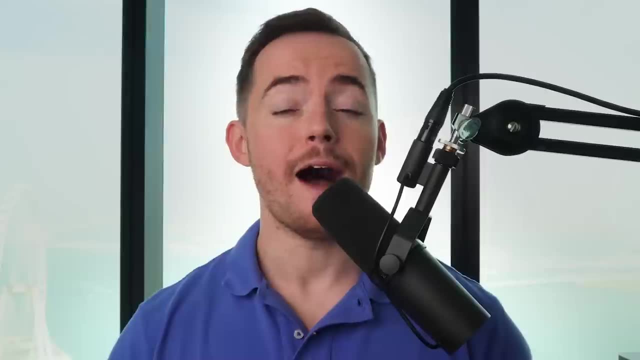 but the face will often become puffy or swollen in appearance. Now this is often accompanied by a slight reddening of the face due to dilation of the blood vessels. Alcohol also impacts your skin's ability to neutralize free radicals, leading to premature aging. In a nutshell, your face just won't look as healthy. These are the early, more acute effects of heavy drinking, But over time these will give way to more permanent facial changes. These include the formation of forehead lines, crow's feet, puffy eyes and, eventually, loss of cheek volume. 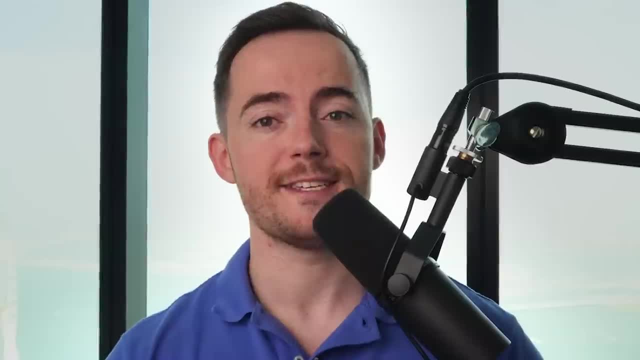 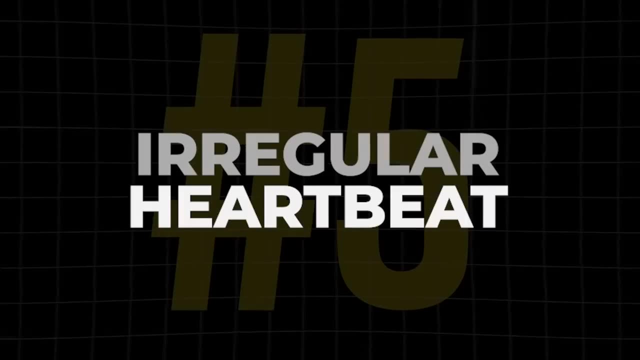 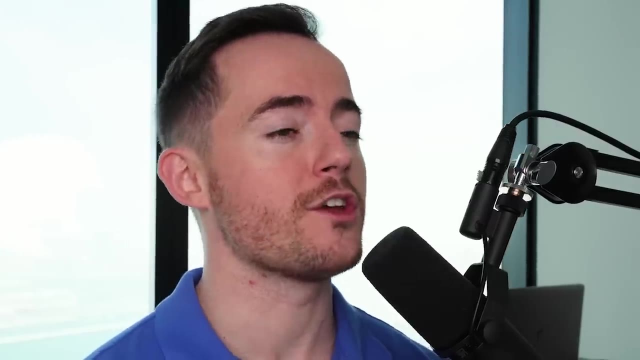 In other words, you start off with a puffy face before progressing to the complete opposite: loss of fatty tissue. This can make you look several years older than your real age. The fifth sign is in an irregular heartbeat. Now, ethanol is a so-called cardiotoxic. In other words, it's toxic to the heart and cardiovascular. system. We saw earlier how it leads to an increase in blood pressure which affects more or less every part of the body. But the damage goes beyond that. When our bodies break down alcohol, in the first instance they convert it to a very dangerous substance called acetaldehyde. 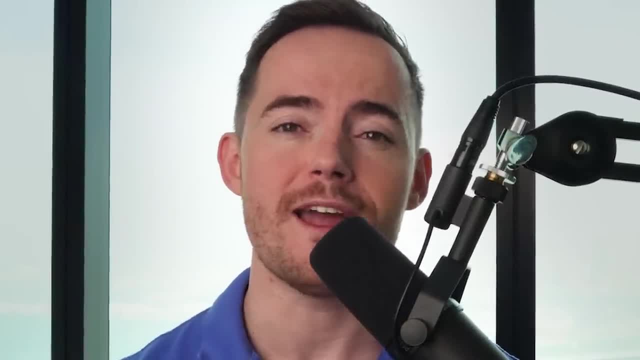 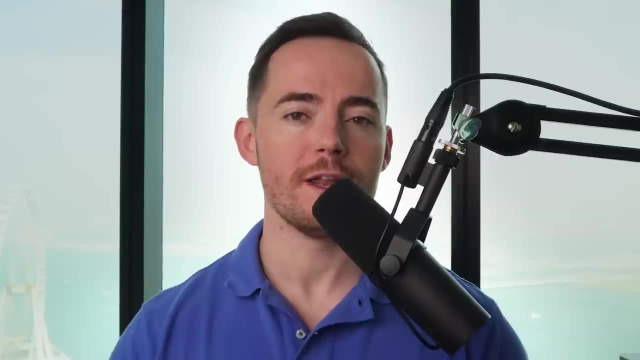 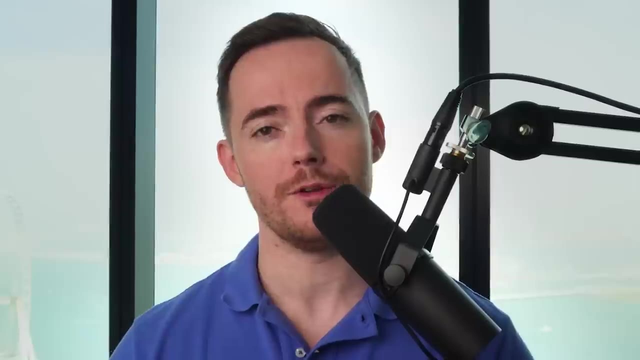 Acetaldehyde is even more toxic to the heart than alcohol itself and directly attacks the heart muscles. Over time this can lead to a condition called alcoholic cardiomyopathy. In alcoholic cardiomyopathy, certain heart muscles literally enlarge and stretch so it has trouble pumping blood. Think of it like a rubber band that's been stretched. out too much. Up to 30% of heavy drinkers seeking treatment in addiction centers do have this condition, And it's tragic to say, but unless they stopped drinking, most of them would be dead in a few years. Maybe something to bear in mind the next time. your evening. news tries to brainwash you about the supposed heart-protective effects of red wine. However, cardiomyopathy is generally a late-stage symptom. You need to be drinking for years or even decades to get there. Perhaps the first warning signs that you are on your way to.